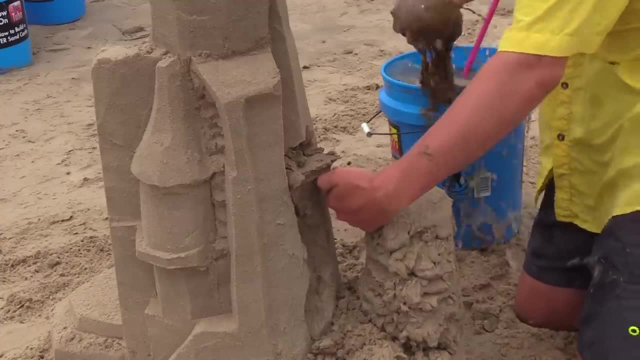 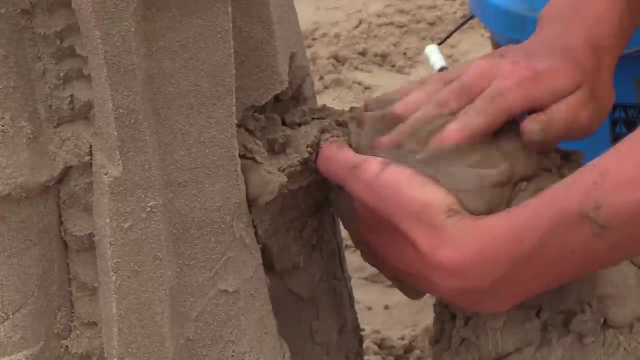 and then he literally just digs the sand out with one hand, just flops it on. and there you go, holding it with his hands, and then he's just flopping it on that bridge, boom, and that's what he does. just makes it a bit thicker, and then he's going to hold it there and just join it in bit of. 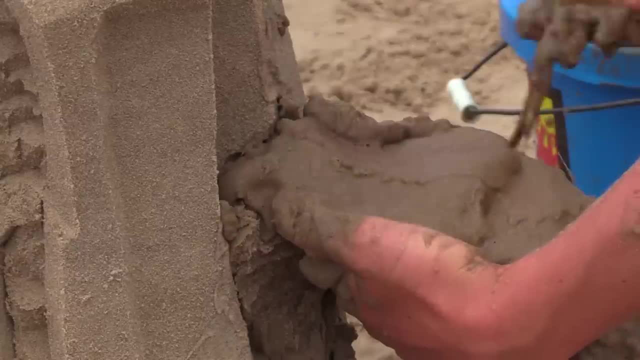 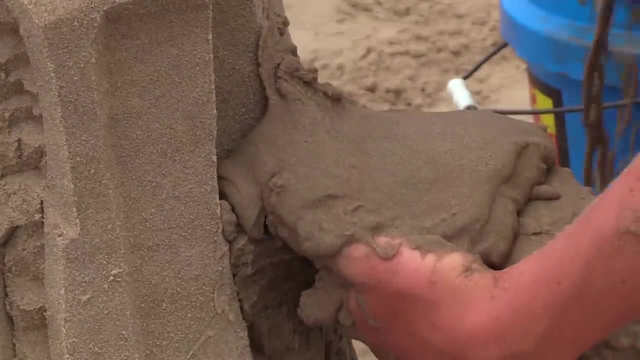 water at the top and then we're going to join that in and make sure that's better and it's just a bit thicker at the top. but that's how you do it: you just hold it with your own hand, use the other hand to lift sand and water out of the bucket, and it just makes it a lot easier. So I'm going to 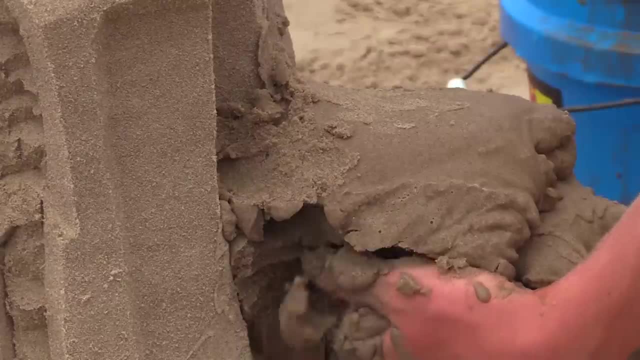 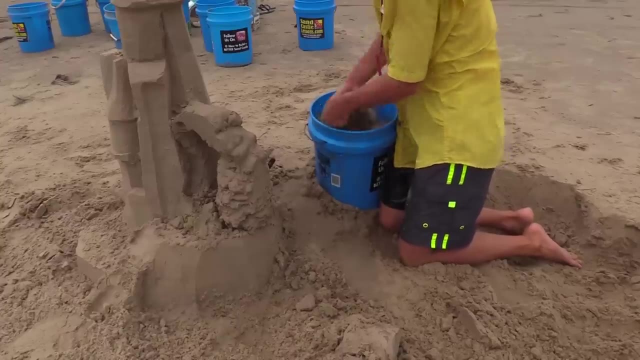 show you how to do these, and if you push the sand and water into the surface, it means it's joined more effectively. So there's, that's exactly how you do hand stacking when you're making a bridge, and then Max is going to join it by literally doing the same thing again. he's made a bit of. 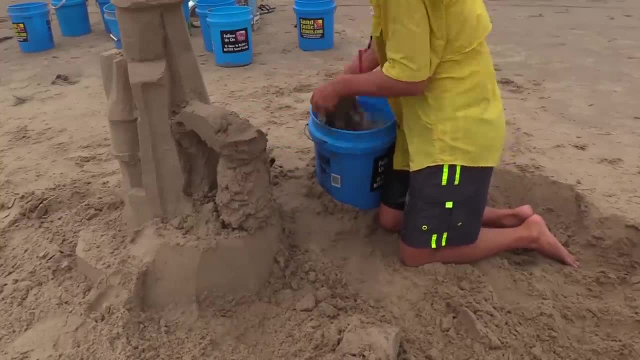 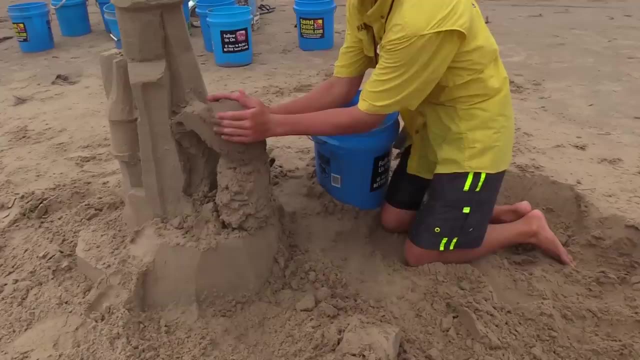 an overhang on that bridge, making it smoother on the top, and then he's going to move down to the down to the floor, I think, and make another bit, but he's going to stack up a little tower first. so there we go: he's making a little tower. 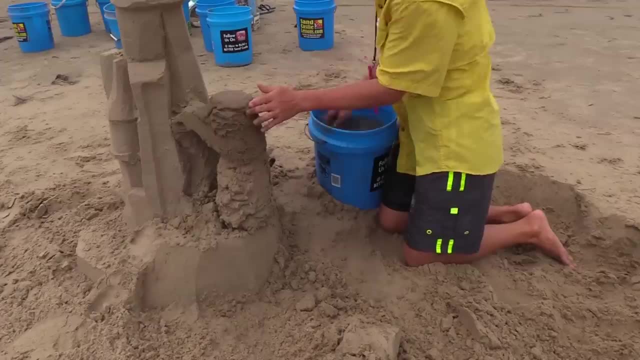 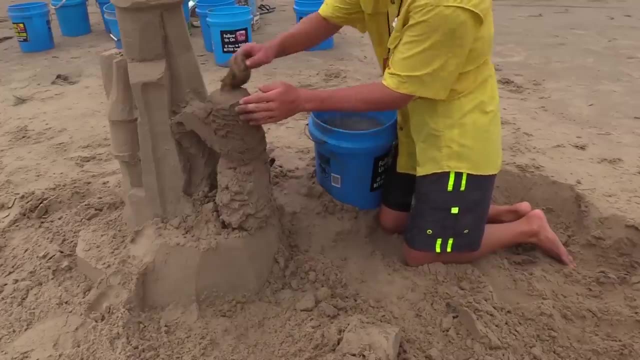 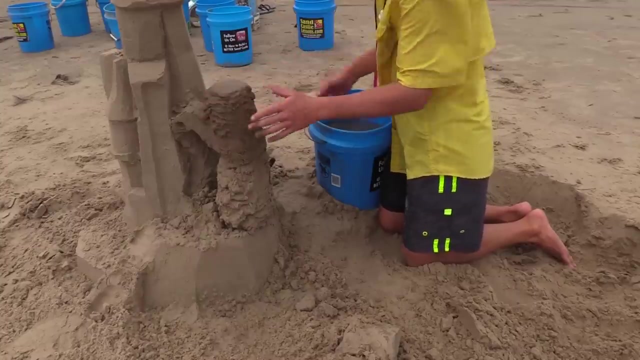 on top of our column, of our bridge, like a little guard tower to change the shape. we're changing the dynamic. we're making the castle look like it's spread spread out all over the place and you can't possibly tell now that it's made from a bucket or two buckets. okay, um, so we're using hand stacking to do something. 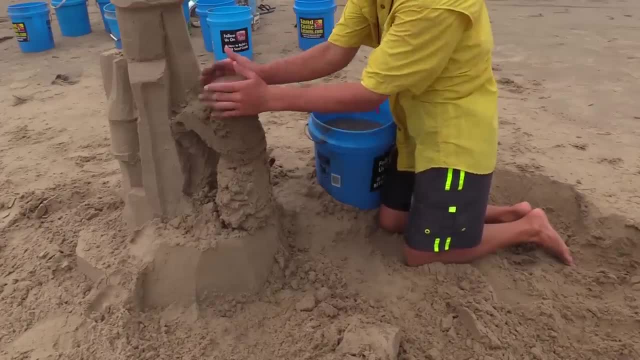 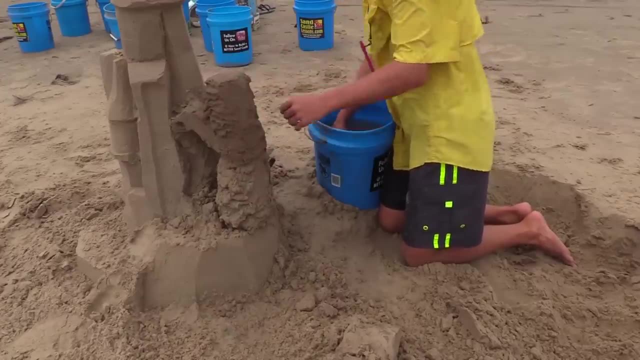 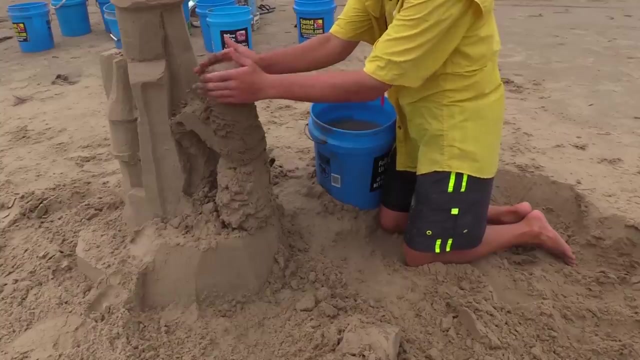 different. the other thing is, hand stacking is one of four methods. there's drip castling, soft packing, hand stacking and forming. they're the four different types of sand castling. so, um, and through the videos you'll see each one. but so at the moment we're doing hand stacking and we used forming to make the buckets, and when we 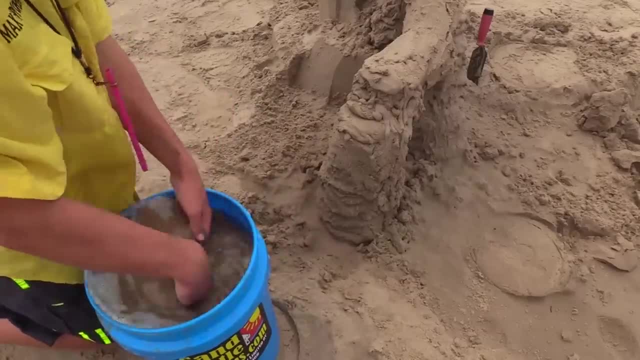 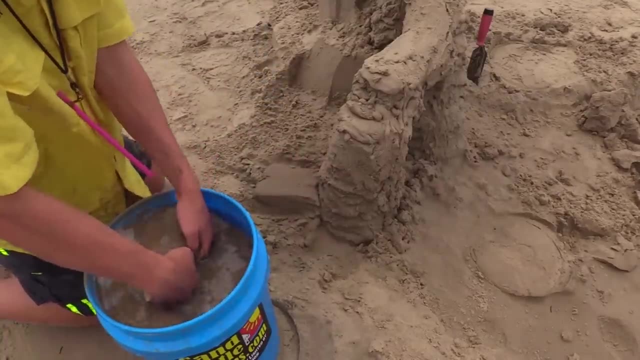 filled the buckets, um so, and we use soft packing when we make the moats, so. so if we want to do a staircase that comes off our little tower, we've done another tower here. we've jumped a bit. we've done another tower and another, another bridge. so what we're doing now is showing you how to. 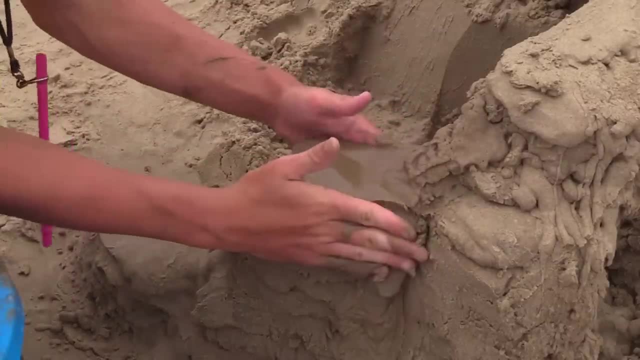 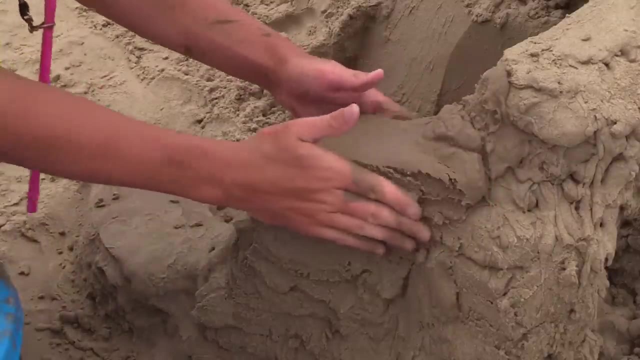 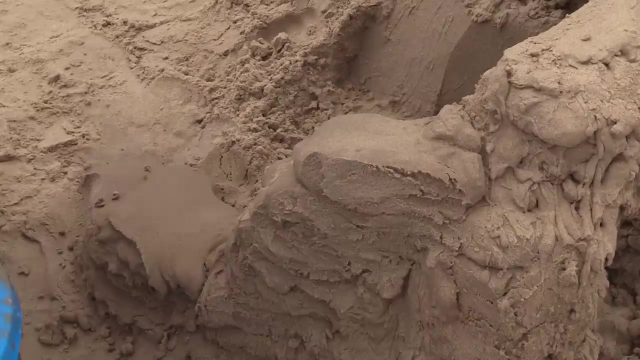 hand stack because, as I said before, girls shimmy and boys jiggle. so we've shimmied all the pancakes on and you hold your hands parallel and you just stack up blocks of sand- really easy. boom, hold it till the water disappears. there you go another one, join it on and really push the sand into the 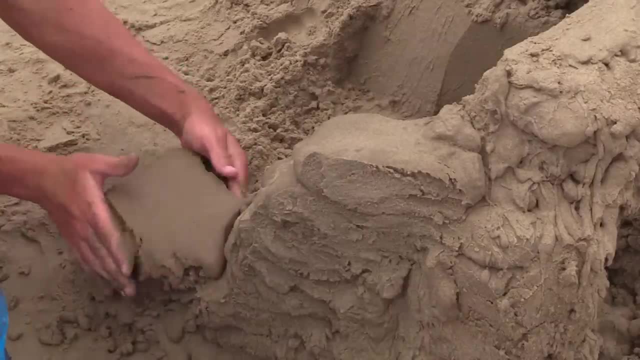 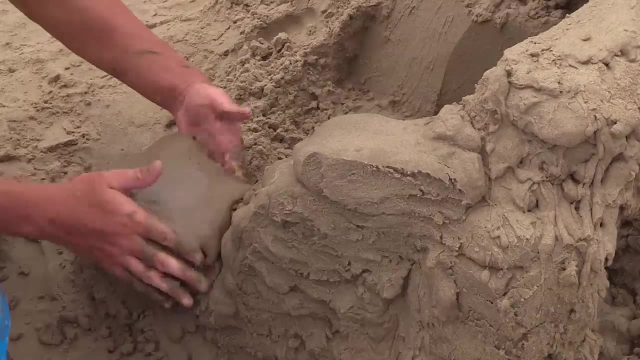 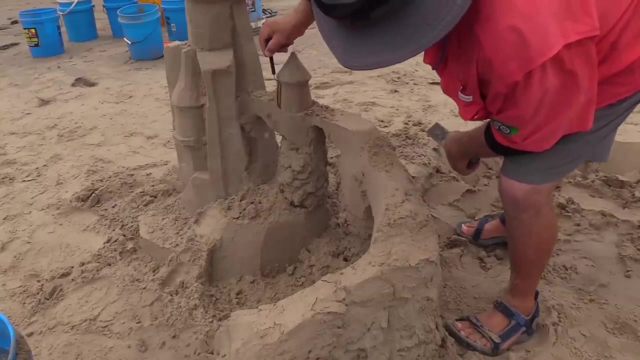 surface of the one up front or next to it, because the water will enable it to bond better. so Max is stacking these away so you can see how they're stacked up together in like an arc and then, after we finish building, all the all the hand stacks. 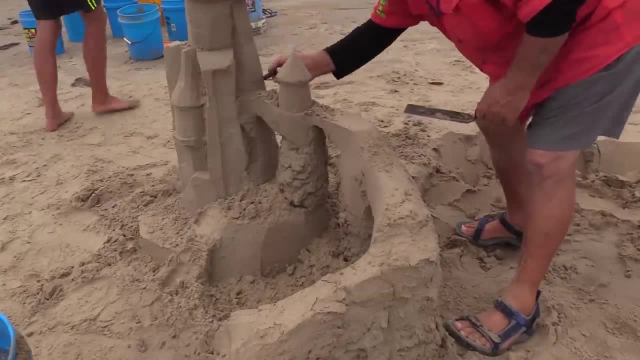 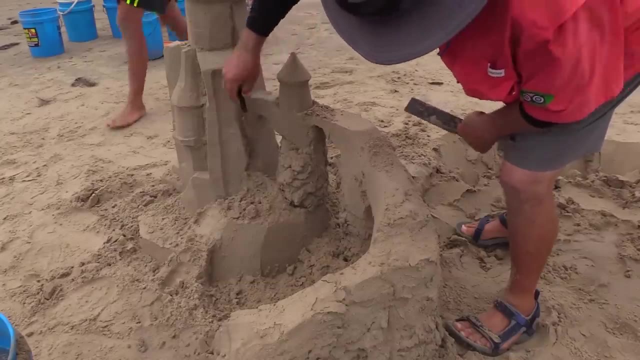 we actually carve it away, so um and uh. so you can do this by just joining it to the castle, making it nice and thin. one of the things about thin bridges is that people go: wow, that's, I mean, how did you get it to? how does it join? well, it's very simple. you have to hand stack it. um, I can show you. 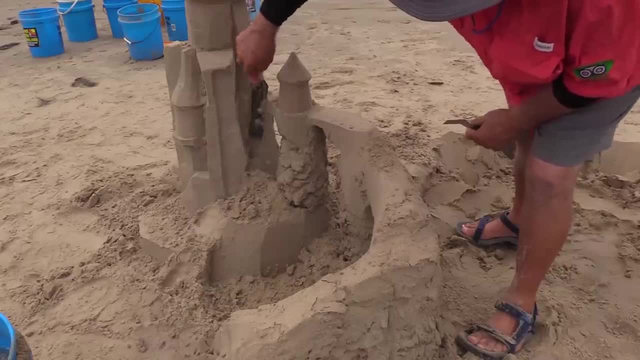 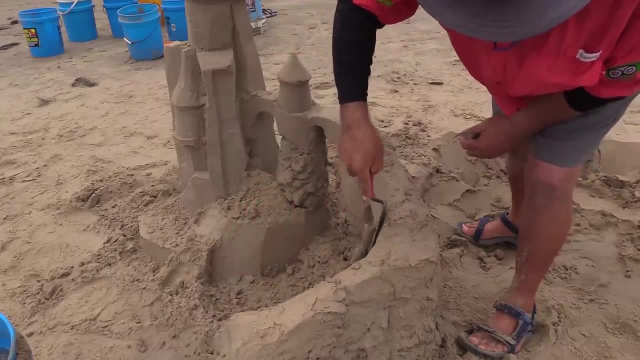 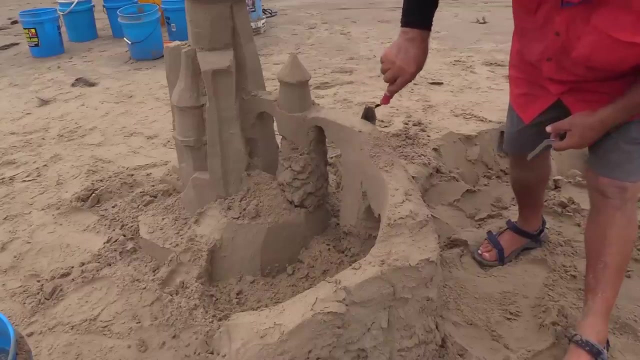 how to pack sand into buckets all day, but that won't help anybody. what we do is we, we um uh hand stack to join elements to our castle that you can't use a form for, and then it gives you a whole new dynamic. people are going: wow look. 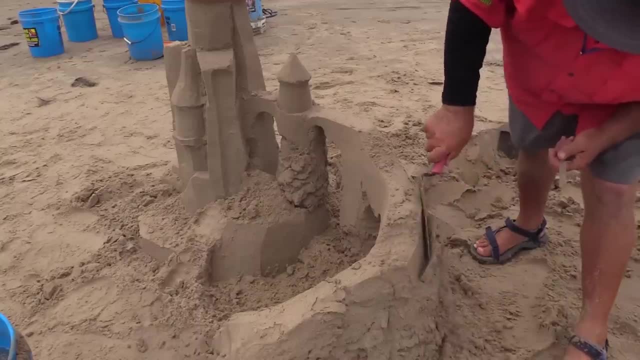 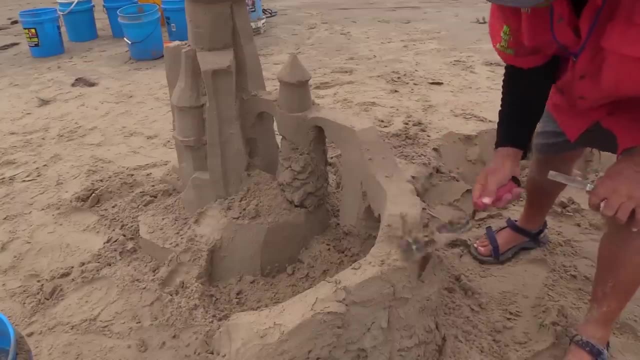 at that. what? how do they make it, Kirby? well, this is how you do it. you actually stack it in whatever shape you want, and then, in this particular case, we're transitioning from one level to another. so we're going, we're going to go down, then we're going to go flat, then we're going to go down. 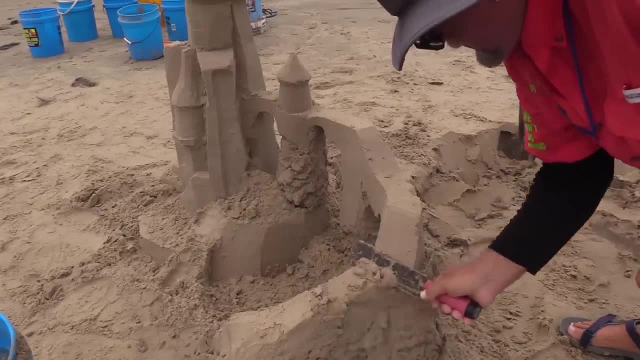 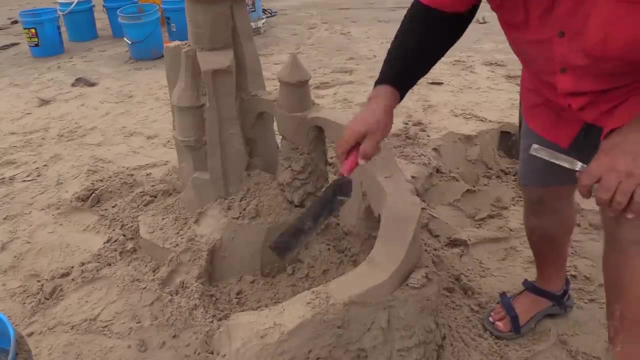 then we're going to go flat, then we're going to go down, so it's just a really easy way to do it. the big spatula is great for doing beautiful flat curves, or big, um, uh, smooth curves, should I say, and uh, and then we're going around at the bottom. I unfortunately didn't film this very well, but you. 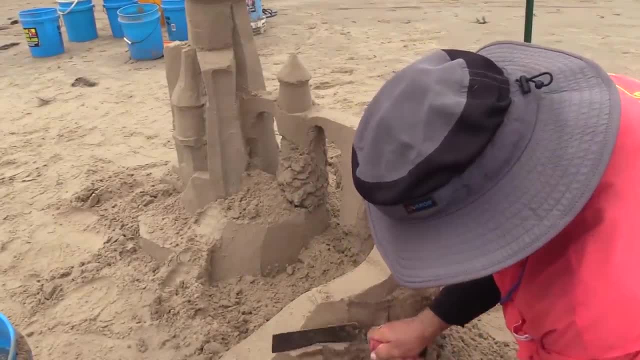 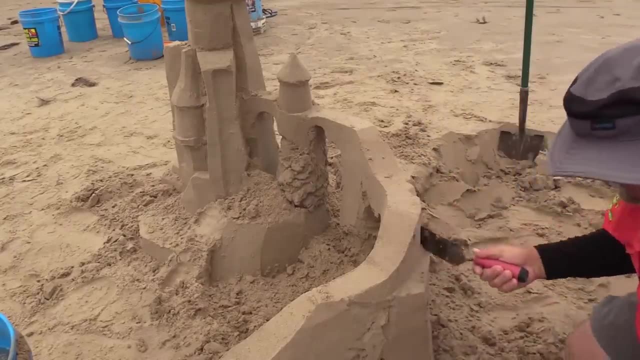 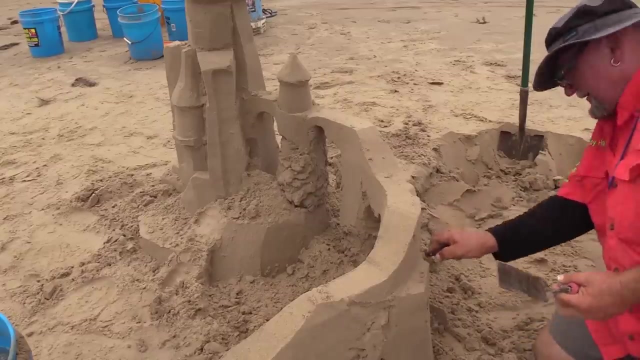 get the idea. so, um, we're going down like this and we're going to make another building here. why not? why not? we've got enough room, let's just make a parapet or a building. a parapet is, uh, something that holds part of a castle or a part of a bridge. so there we go, and now you get your small spatula. 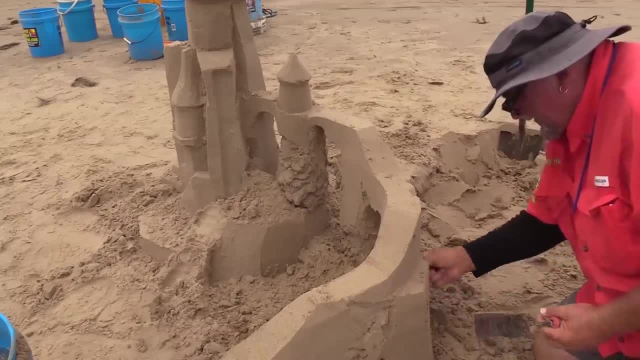 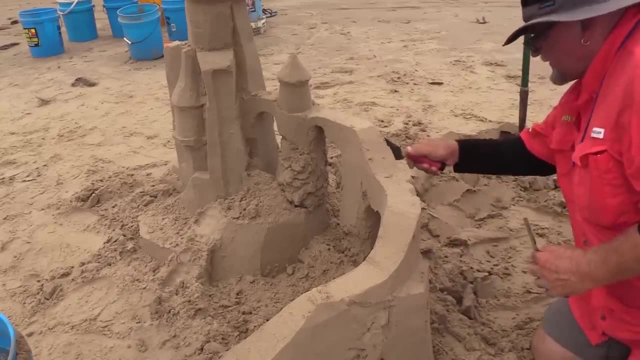 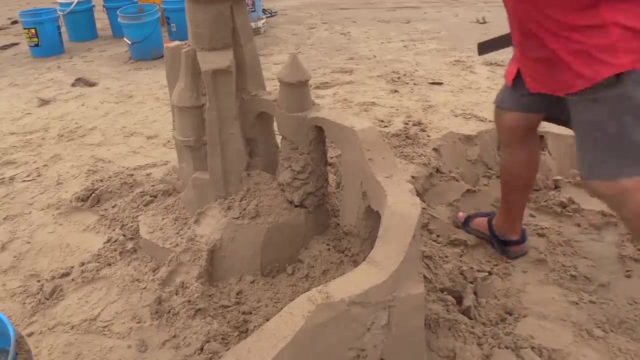 change spatulas again from large to small, oh, and then from small to large. large is great for doing this, flat sides and for doing the sides of the of the support columns. um, like this makes very beautiful big flat cuts and we like that. so then we move around and I think now we change spatulas again. um, yes, there we go and we now do the bridges. 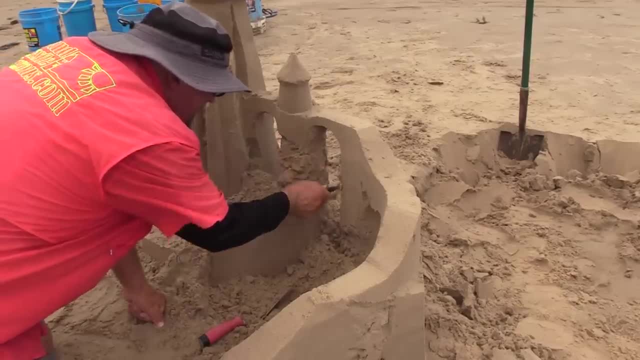 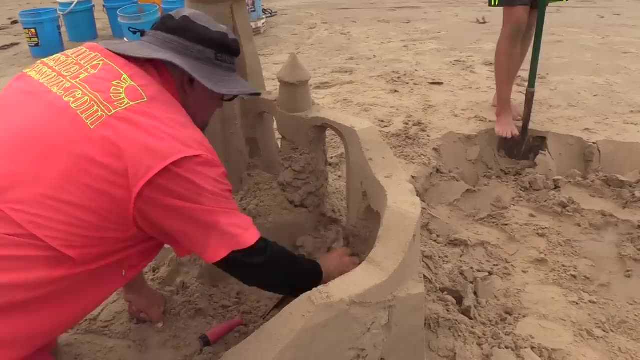 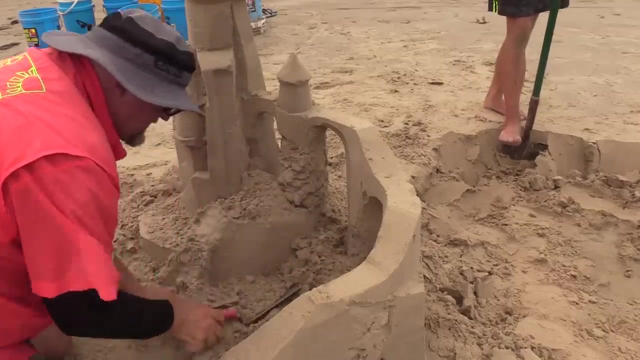 nice and thin using our small spatula. um, there you go, and then we can put an inset in it by using a little offset. remember the offset. the little, uh, the little bend in our spatula makes these beautiful um shapes. then we'll pull that out and we'll get the side dead straight using our really big spatula. 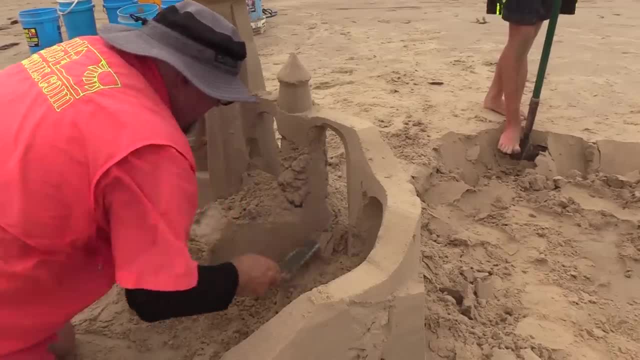 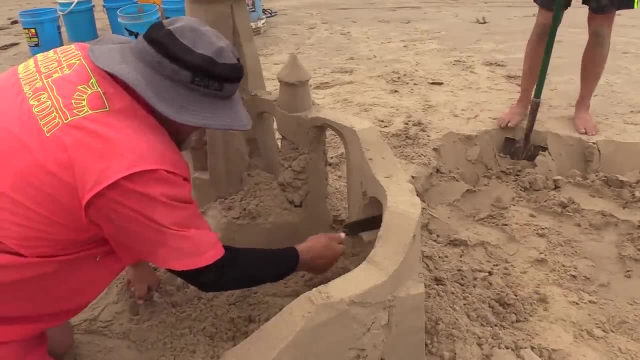 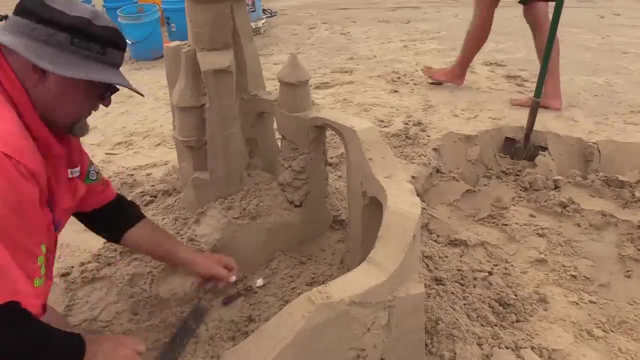 which makes it very easy to scoop things out of the middle and and do that. so this is, this is where it gets easier. um, because we find that we can do all these different things with, um, uh, with the two- just the two- spatulas. so this is why we're making these videos today: to show you how handy this can. 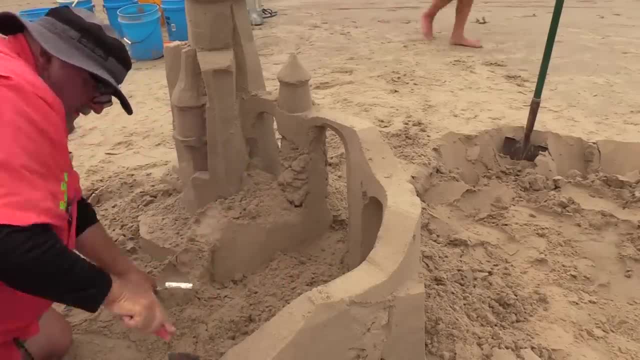 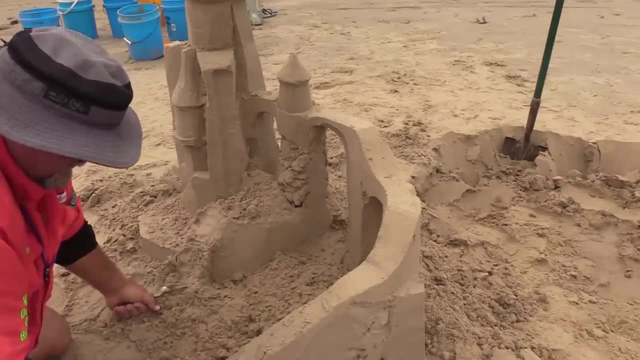 be. and now the tools obviously we sell on sandcastlelessonscom. uh, trowel is something we've got a new now. so, and you don't get it with your lesson either, you have to order it specially. so if you are going to book a lesson and you're watching the videos, make sure. 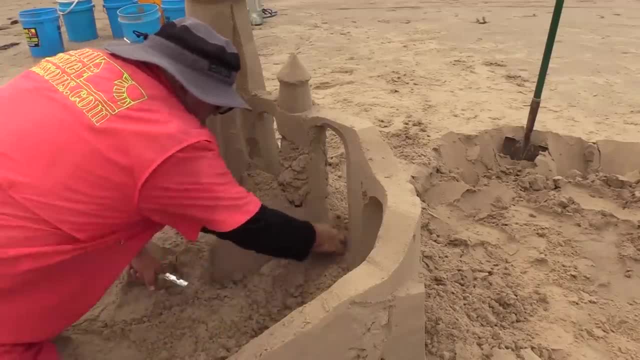 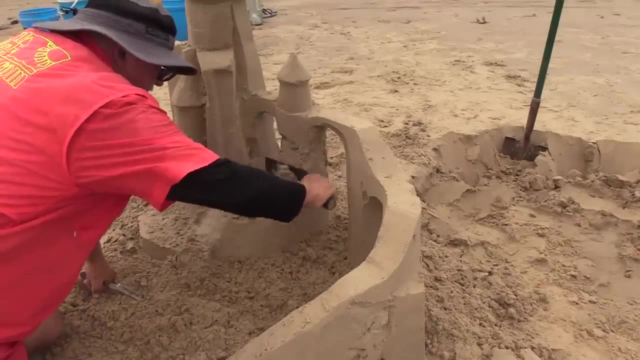 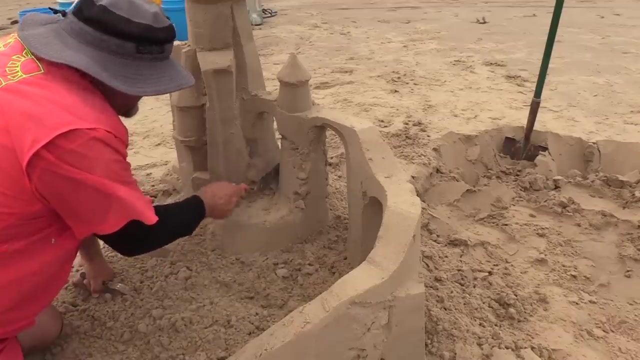 that you tell us you want the extra big one. it is available on the website to order. so, again, keep it smooth and then, um, just pull away all the rough debris and then keep your tower smooth and your debris crunchy, as it were, like rough, and then, if you do that, what that will do is give you that. 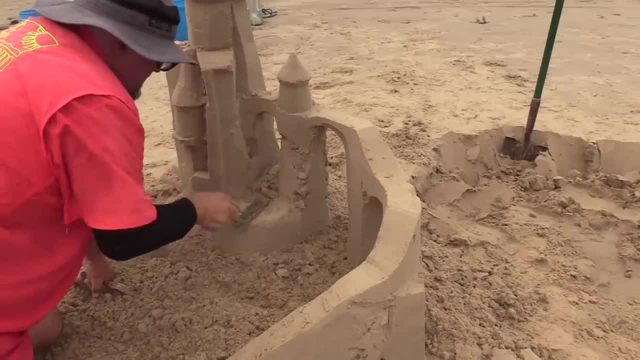 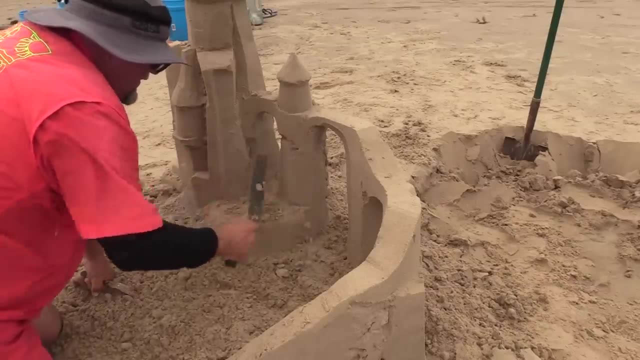 lovely contrast which makes your sandcastle pop straight out of the beach. it's like, wow, how did they make that come out of the beach and get it so smooth? so if you do the smooth bit first and then add the sand for the rough bit, you won't have a problem. oh, change. 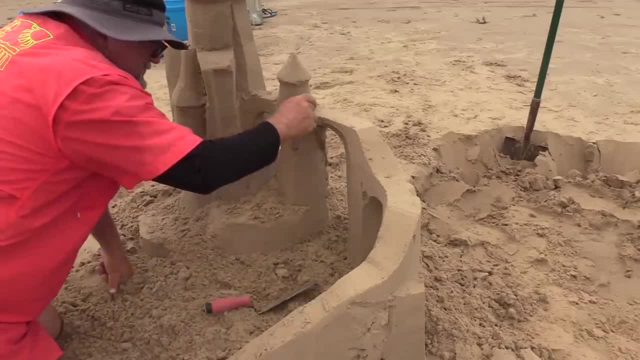 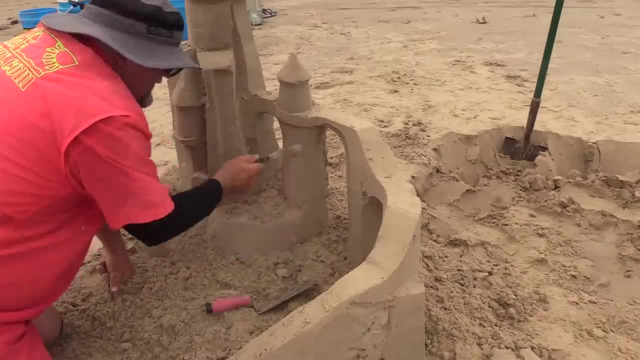 bachelors again and look, we're going to go around and make that walkway, go around that little tower, and then make it smooth and then carve that, so it's a nice smooth column. okay, and we're not, as I say, we're not- doing any decoration today. what we're doing is showing you. 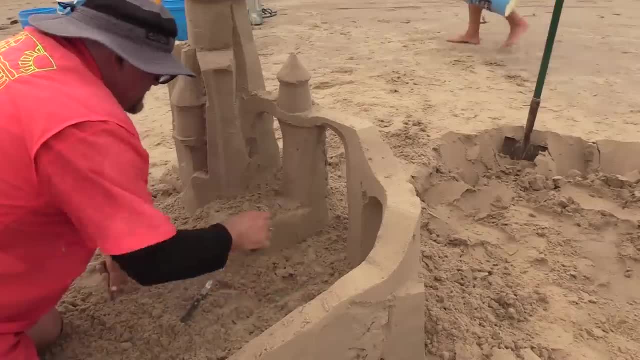 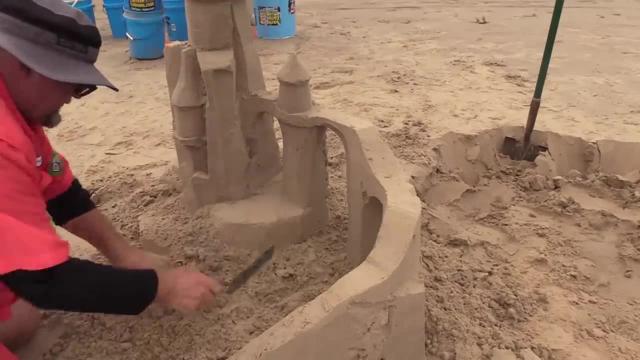 how to use the spatulas. so it's very simple: get used to your big spatula. I mean, if you do go to the beach or you've got a beach location or you go for the summer, it's it's worth investing in a big spatula because you'll be able to do anything- everything- so much quicker. 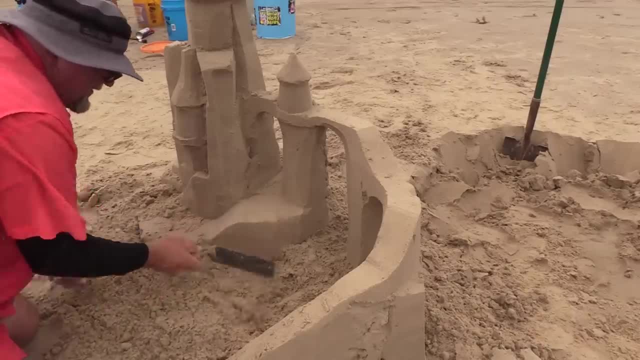 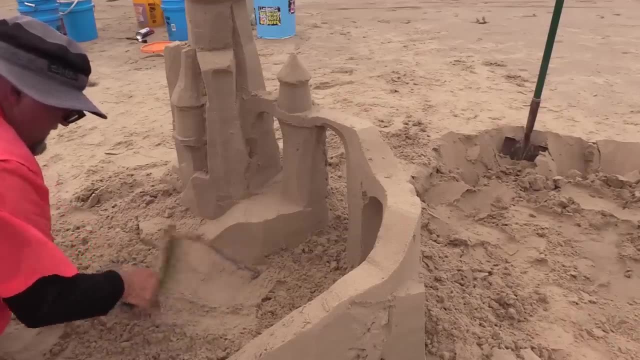 um, and then so we're making it go around here. so we've got like another courtyard and we've got some more, got some more water and we're going to go up here and have set of stairs that go down to the water and the water would obviously have a boat by it. so you know, away we go. so 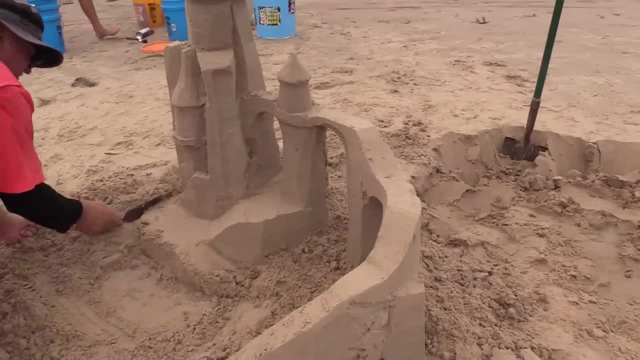 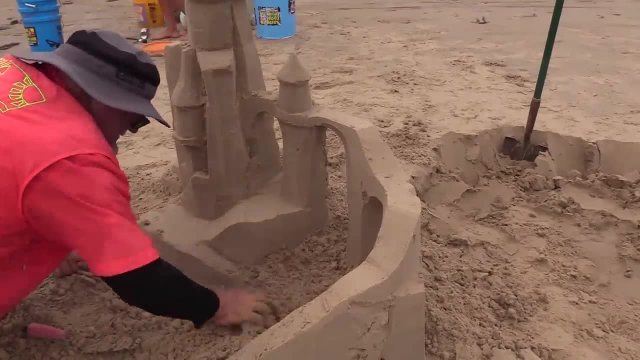 and do that, and then we can go around and you know. so. hopefully at the end it doesn't look like a bucket. so that's what we're doing. um, a bit more spreading: use your hands- one of the things about raking with your hands. raking with anything, it shouldn't look like a rake when you finished. shouldn't be any rake marks in. 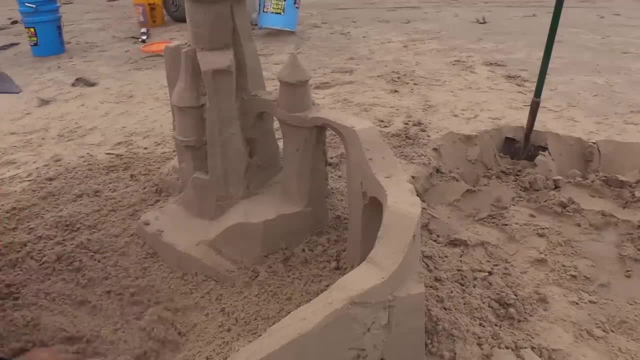 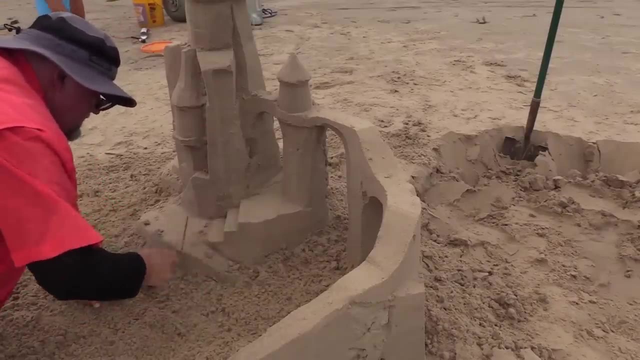 it, so it should look scattered, um, and that makes it really effective. now here's some big steps using the big spatula, and people are always very concerned about steps. oh, i don't think they're up to code. you know whatever that means. who cares? if they're up to code, it's a castle. so we're doing. 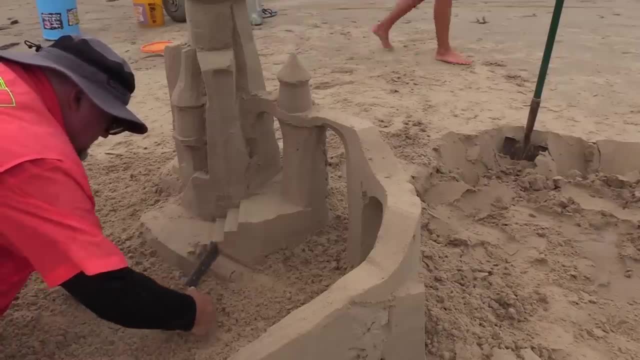 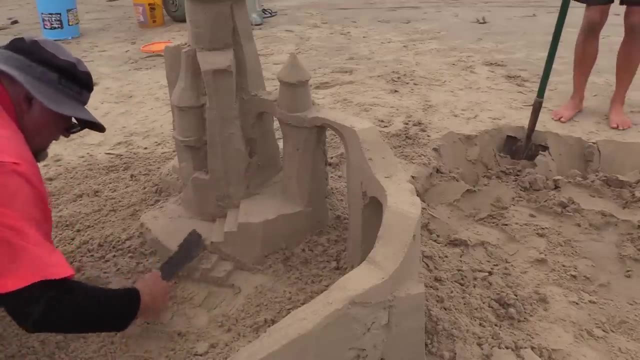 big steps and showing you how to do big ones really quickly with the big spatula, which is very fast like that. so they they then go down to the and uh, yeah, all right, so they do that and spread them out and do all that stuff, and then then we can use the small spatula to come in and 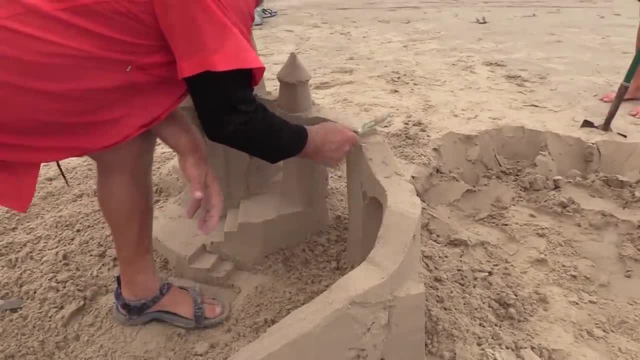 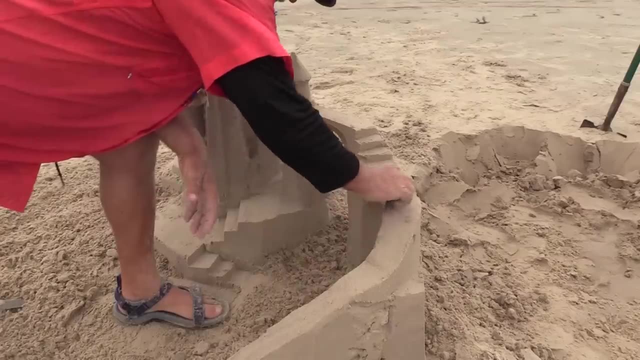 do smaller steps, they're still quite big. yes, you can make them smaller. i just doing this quickly for the video, but it shows you. you just go keep that flat and then you come around the other side, which we have to do for filming, and then you go down out sideways in. 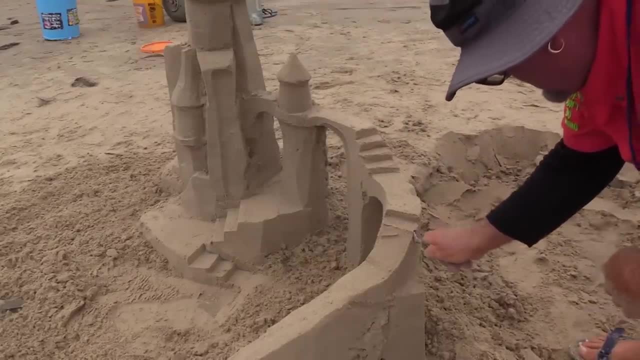 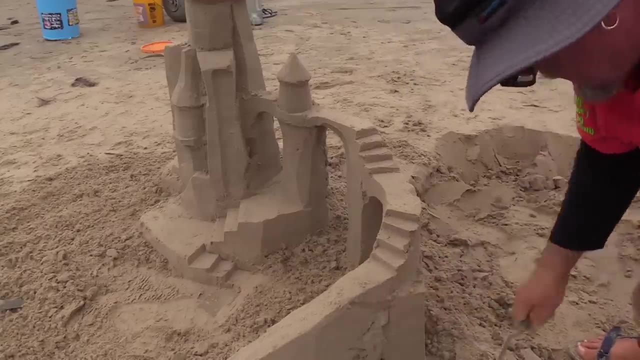 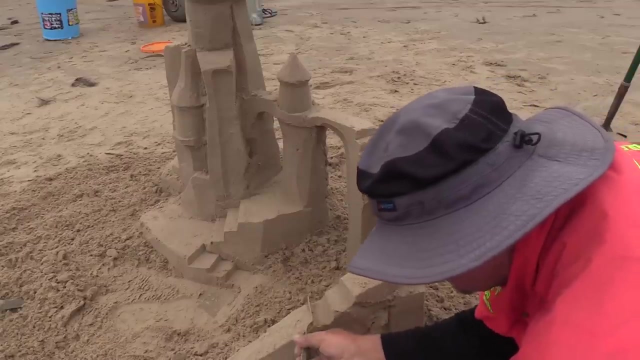 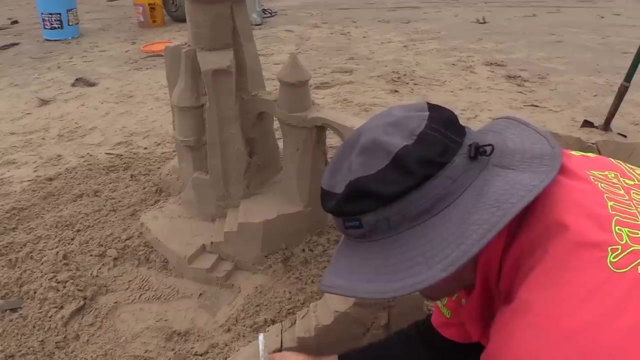 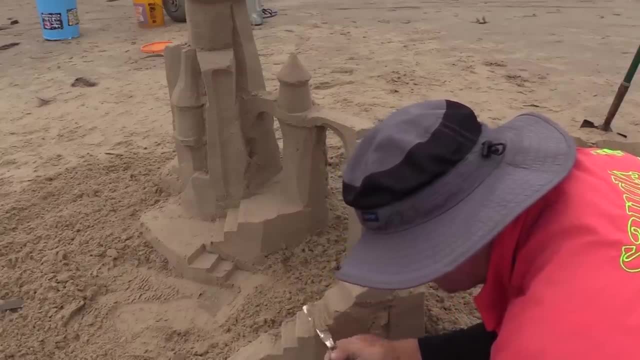 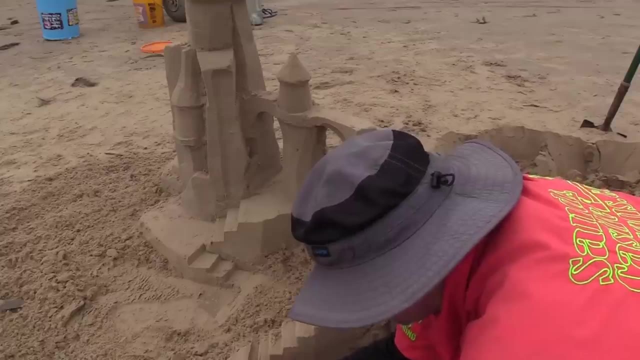 would turn the spatula with it. so we're going to do that, but I don't think this one turns very much, so I think it's pretty straight. so that's how you do that. so my name is Andy Hancock. thank you to Max of Orca for being on the. 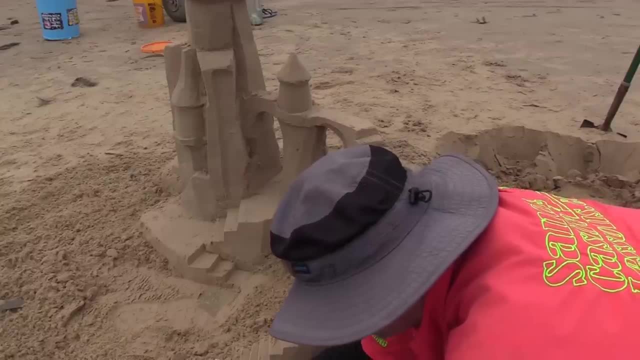 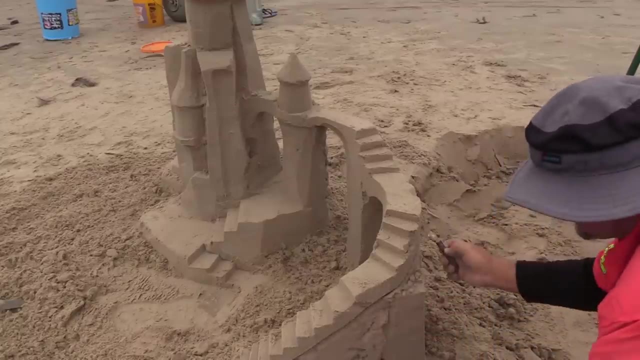 video. he's a great guy and and he's one of the fastest hand stackers I've ever seen. so and then after when you do the the stairs, you can always cut away some of the stairs underneath, so your staircase pops out from the top of your 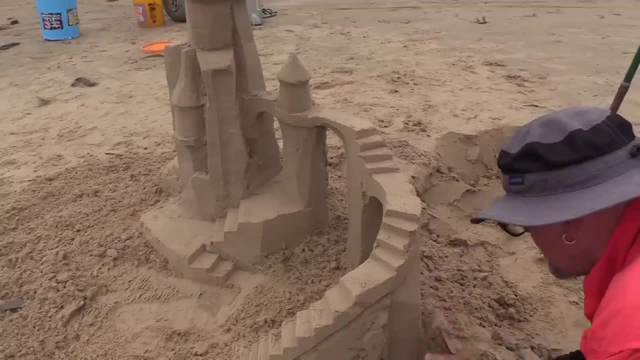 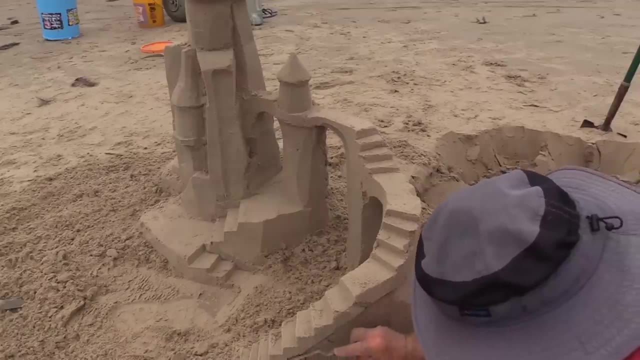 castle and people go. well, why doesn't it just fall off? that's because we're all magicians. it's all smoke and mirrors. okay, so it's not smoke and mirrors at all, it's engineering, it's actually physical chemistry, and what we're doing is forming interstices and doing all sorts.